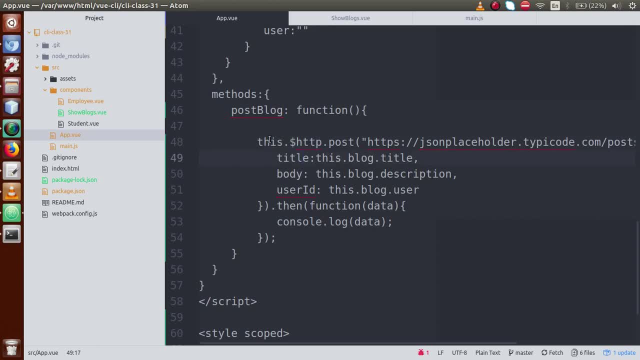 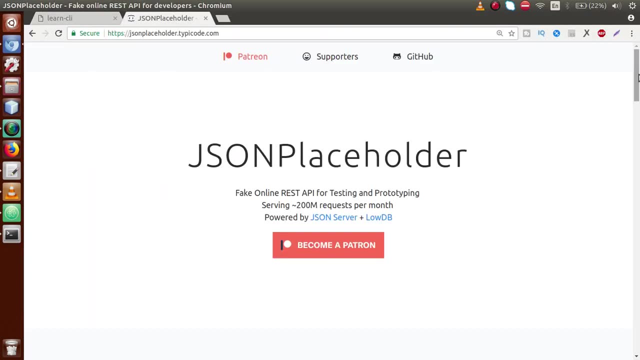 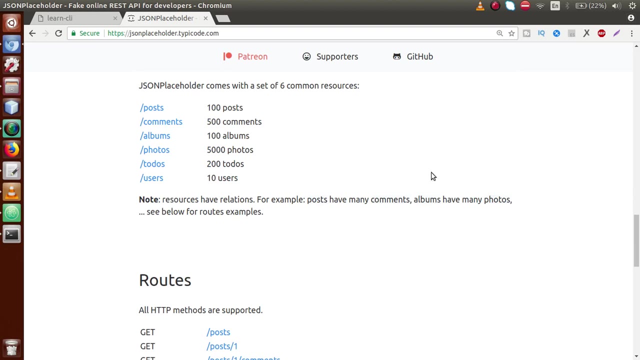 Okay. So basically, guys, now what we are going to do is that we are going to use get request concept. Okay. So, if I go to the browser, This is the website, guys, whose fake JSON REST API we are using. Okay, So, just scroll down. So this is the route guys post which we are using. So 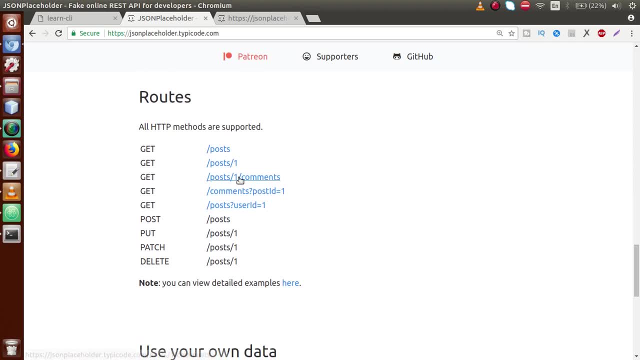 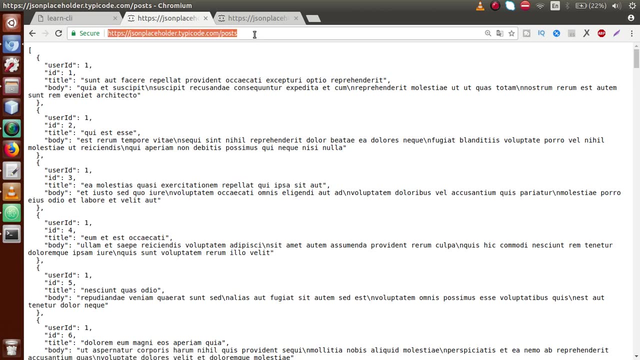 if I open new tab and go to the routes, guys, then this is our get request, Okay, So if I click on it, So basically we will hit this URL by using get request, Okay, And after that we will read the data, Okay. 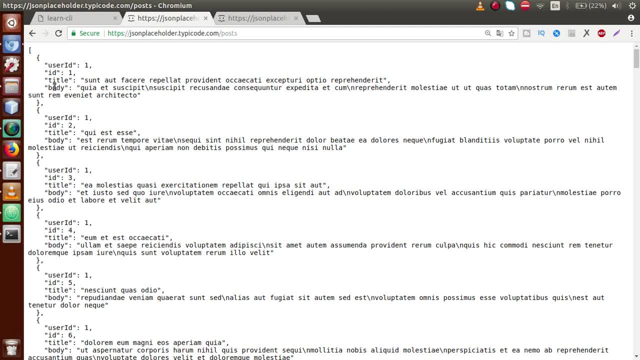 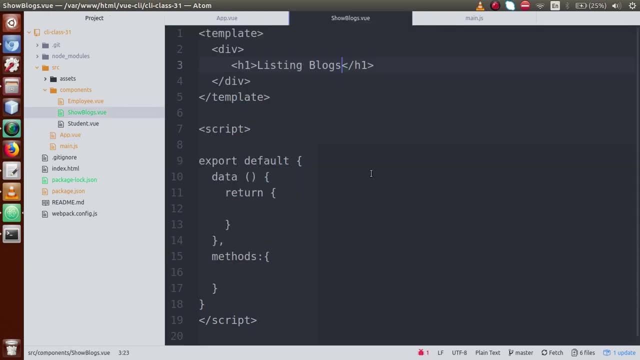 So, basically, as we can see that this is array of objects, Okay, So, where one object, two objects, we have 100 objects like this inside this array. Okay, So just back to editor. So now, what we have done for that guys is that we have created a Vue file, Something. 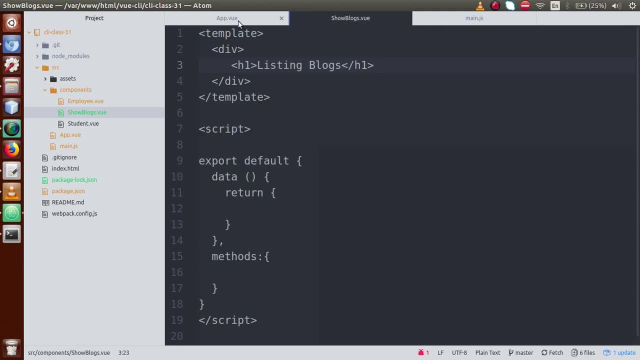 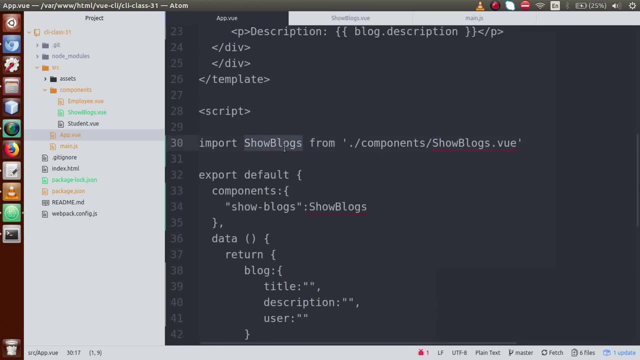 called soublocksVue. Okay, We have imported this block on our route component That is called AppVue. Okay, Here we have imported it And now we have imported it, But we had, After inputting it, we have defined a component and this is the tag to show all blogs. 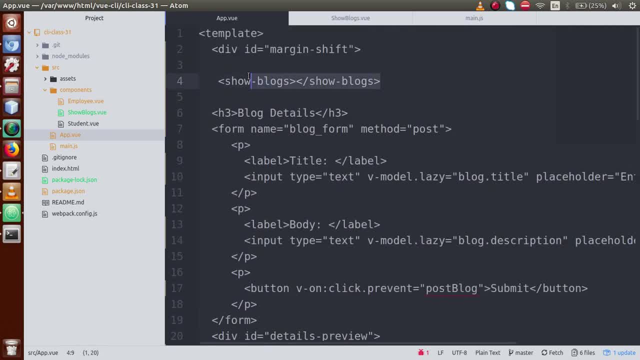 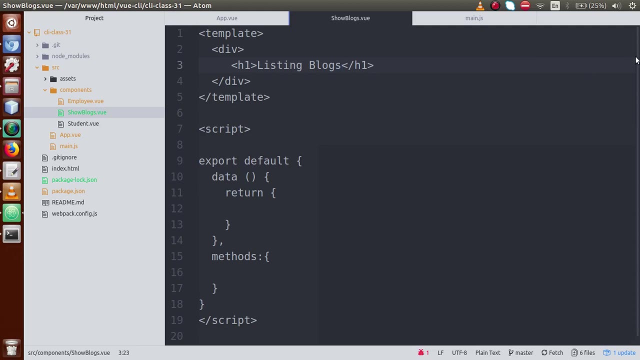 Then we have called this showBlogs, something like here. So if you go to front end, So this is called listingBlogs. This listingBlogs content is coming from our showBlogsview component, So we will read those posts on this file, So just scroll down. 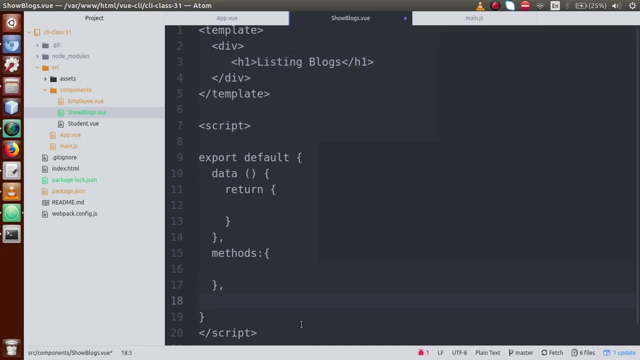 Right here, guys, we will define a method. If you have seen our previous video sessions, guys, Where we have discussed about lifecycle methods, So there we have shown a method called created. Basically, this actually function will fire when our component in slices. When our component in slice, guys, When our component means declare. 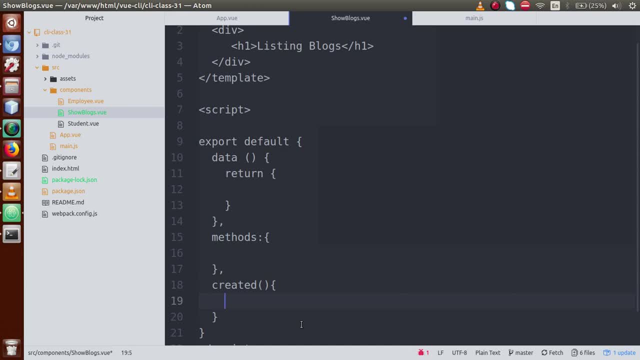 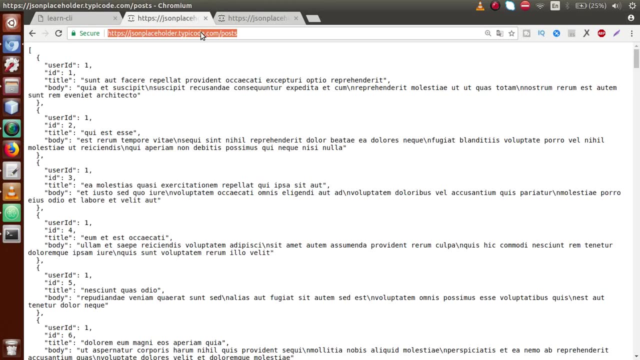 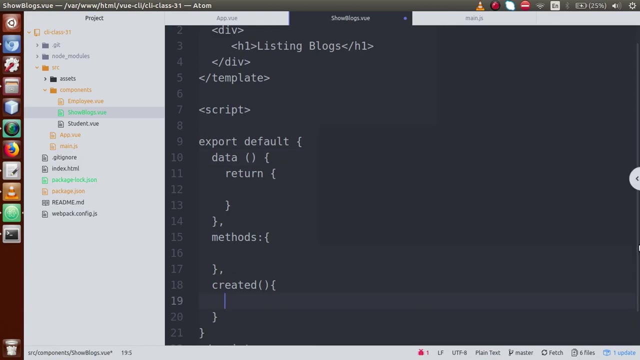 Then this function will fire. So inside this function, guys, We are going to make the get request to the fake JSON registry BI, So I will go Just copy this URL, Go inside this function And let's say that Inside this created function, Let's say this: httpget. 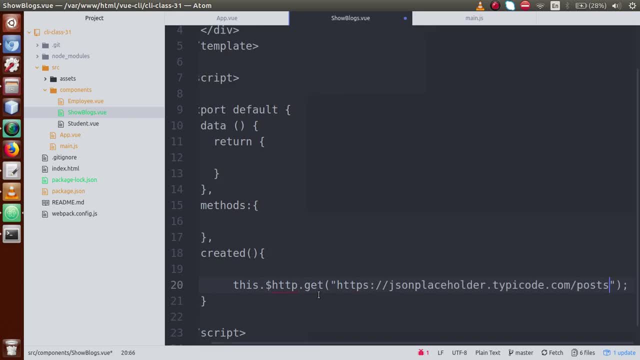 Okay, This is the method, The first parameter which we will pass, guys, That is called the URL. So, basically, guys, here we are hitting this URL instead of the get request. Okay, Now we have to access those data, We have to access that data Which will come. So, basically, we are going to use called then. 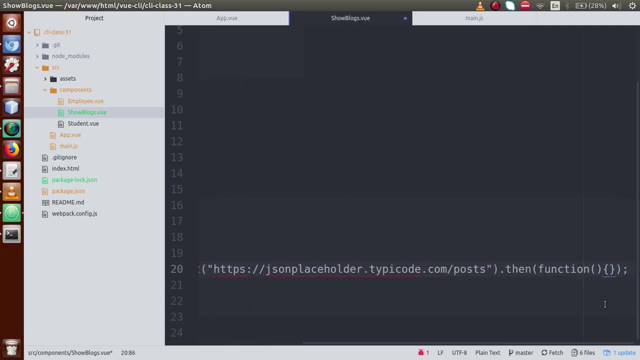 Inside this. then let's define a function And now inside this function, This is the data variable. All those values will come inside this data variable. Okay, So just go inside this block And let's say that Consolelog, And basically we are going to console those data. So let's say data. 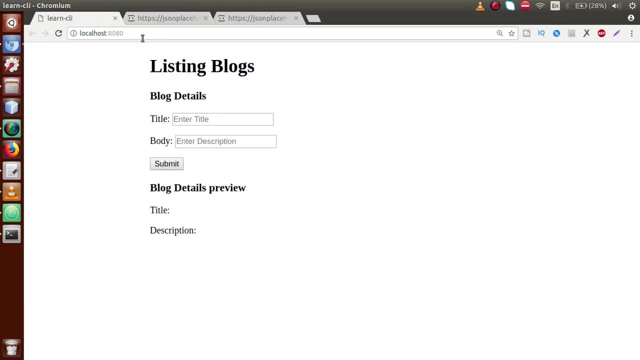 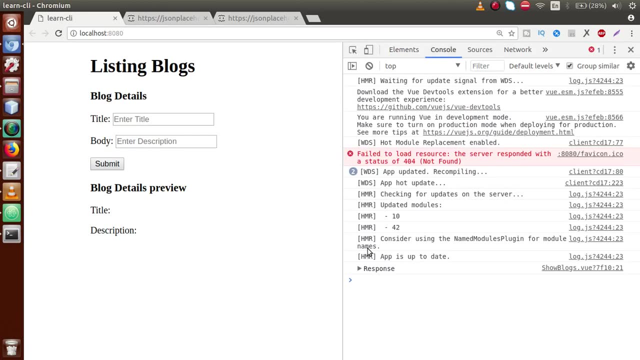 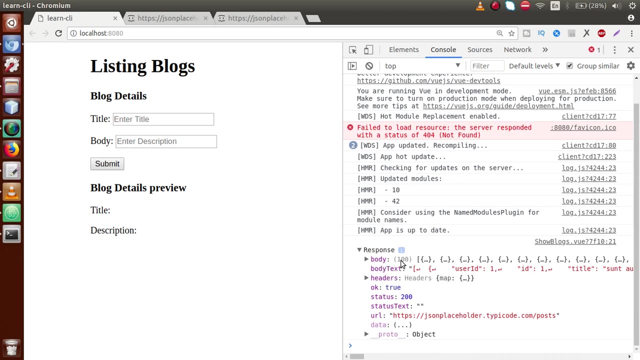 Okay, So just save this file, Go to browser And first let's inspect. Just go to console And now, guys, we can see. This basically came in the response name variable And this response was our body And here those 100 objects. Okay, So, basically, this is an object. 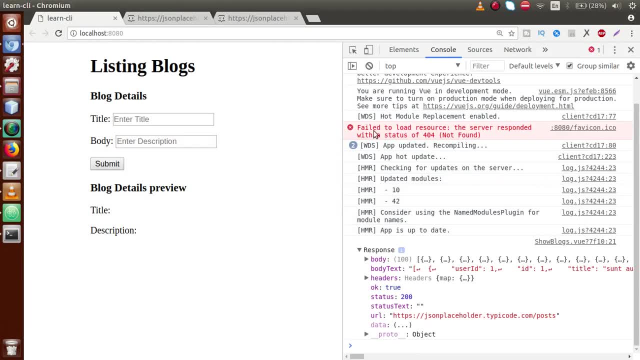 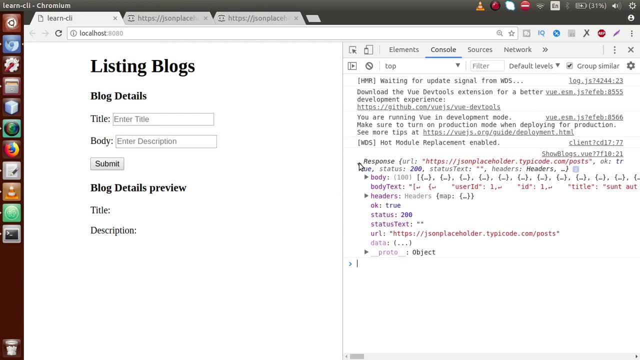 And this is the response, guys, Which we have console. Okay, If I remove this, Just reload this page once more. Now, this is the response. Just open this response. And inside this response we can see, guys, Inside the body parameter, We have 100 objects Which are in array format. 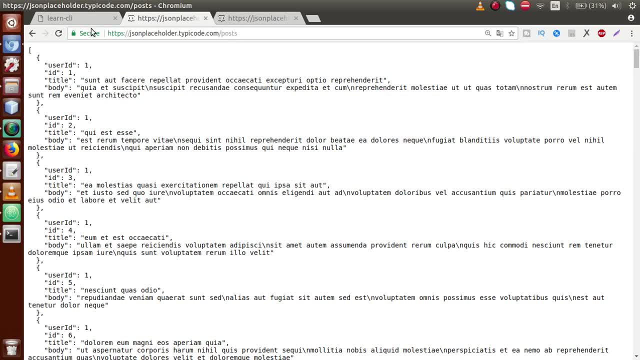 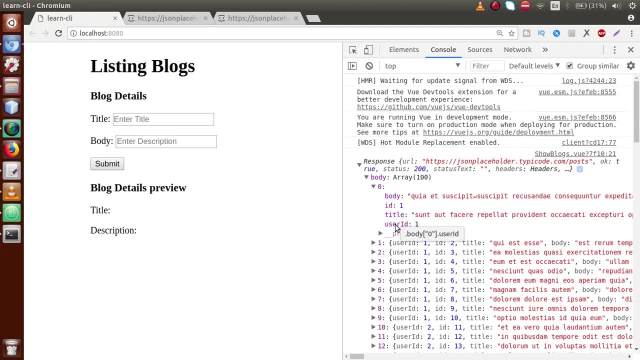 And we have read those data from here. Okay, So basically, it is a single object, guys. Which parameters does it contains, If I open it, Like body id, title and user id? Okay, So these are the parameters That we are going to read. Okay, So just back to editor. 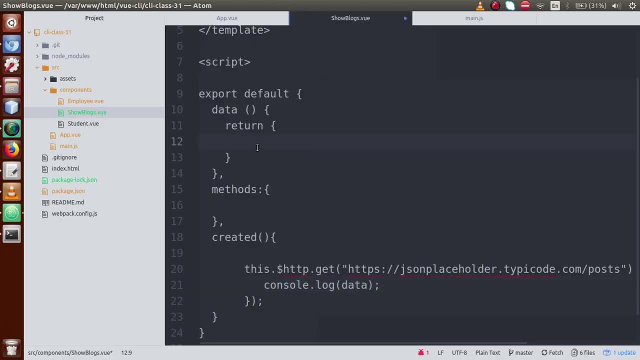 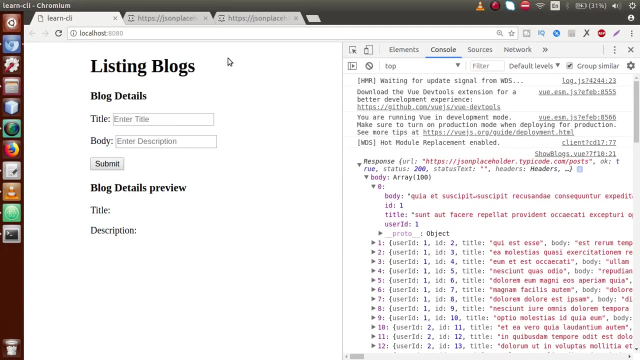 Let's say that I will define a variable Inside this data object, Something called blogs. Okay, And let's say that Data's, So just change it to blogs. Okay, This blog. basically, This is an array. Why this is an array? Because we are getting array, Okay, We are retrieving an array here. 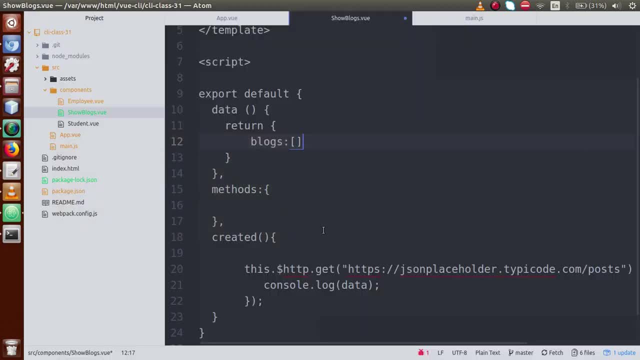 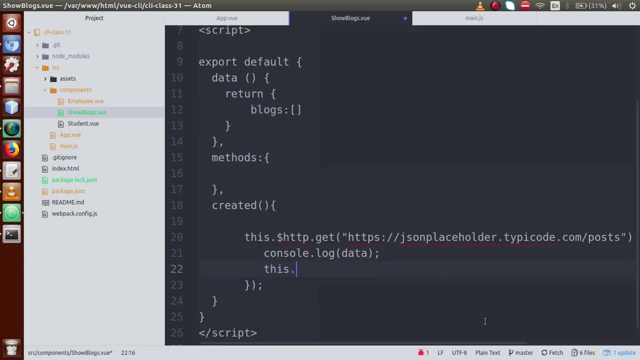 Okay, So basically this is array. After that, what we are defining, guys, Basically blogs, We are going to in slice that variable here. So something called this Dot blogs Equal to something called data. Just copy this data Dot And basically, guys, This response is coming here And the response that's coming here. 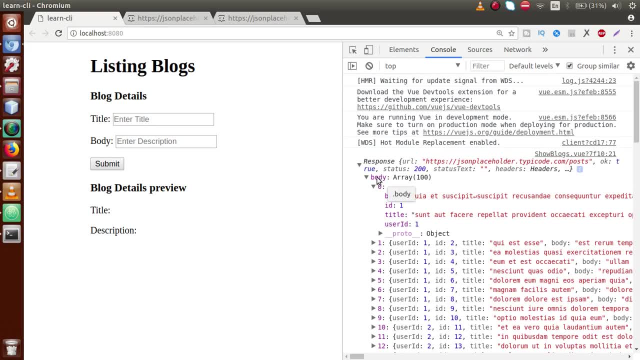 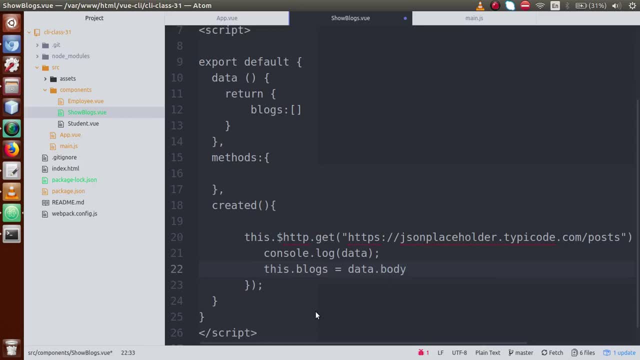 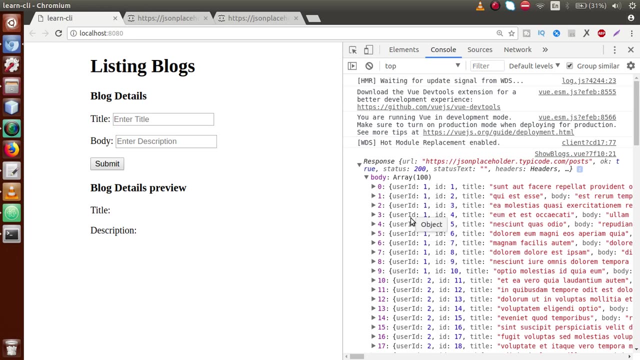 This response is within our body: expert Parameters. Okay, All these values actually stored Inside this body. Okay, So data Dot Body. After that, guys, We are not going to read Three hundred records. Basically, we are going to read Something called five records. Okay, Only five records. So just back to editor. 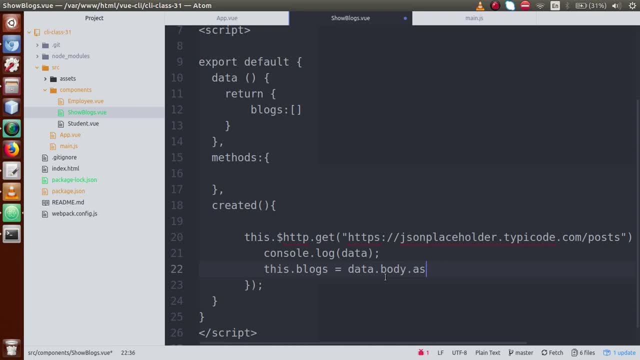 So we are going to use A method called slice. Okay, Slice method To be used, guys. We can fetch five records, Okay. So basically, it starts from 0 index and total size. actually, we are getting called 5, okay, It started from 0 index and total record we need is 5, okay. 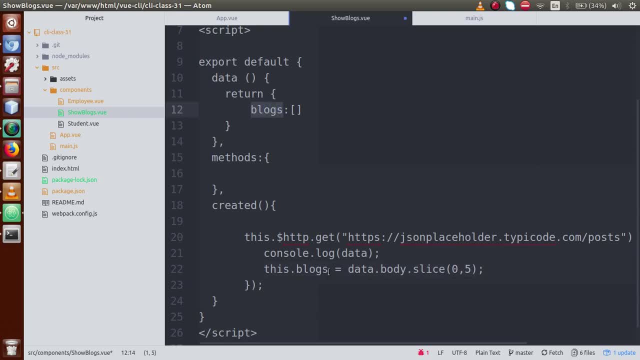 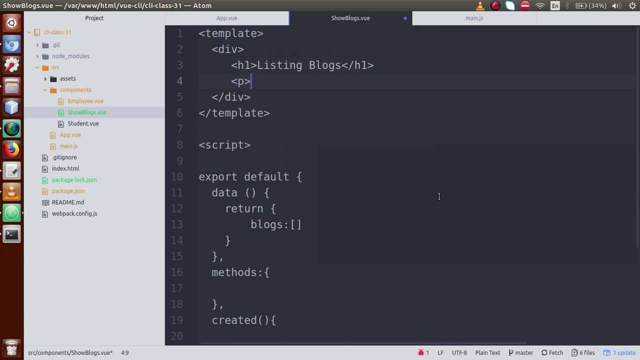 So what we did, guys, In the blocks name array, we have in-sliced the values. okay, Now we have to read this blog right here, okay, So I will go and let's say that inside this paragraph just I am going to use, called v4 directive, okay. 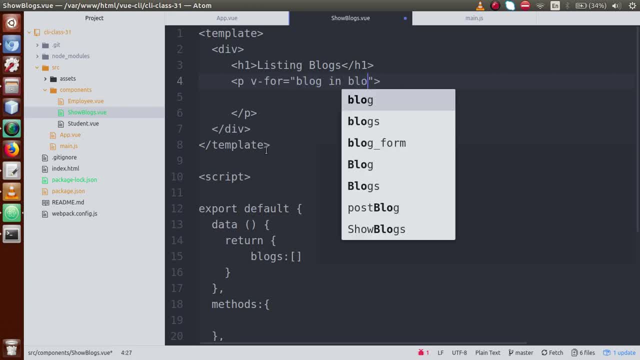 So let's say that blog in blogs, These are the blogs guys which we have in-sliced here. okay, And inside this p, let's say span, Inside this span, let's say that. or instead of this p tag guys, we can use div. 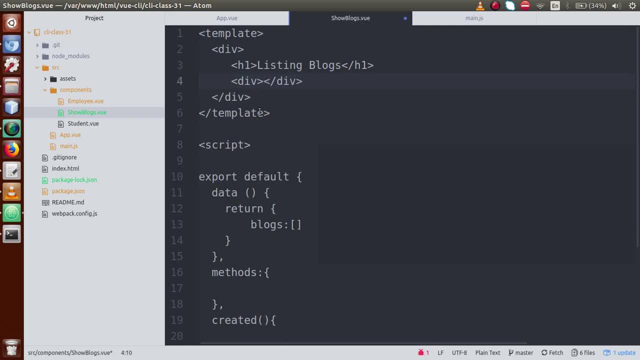 So let's say div. Inside this div, let's say v4. Blog in blogs. Okay, So just inside this div, let's say that paragraph, or let's say that h3 tag. Here, guys, we are going to show the title. 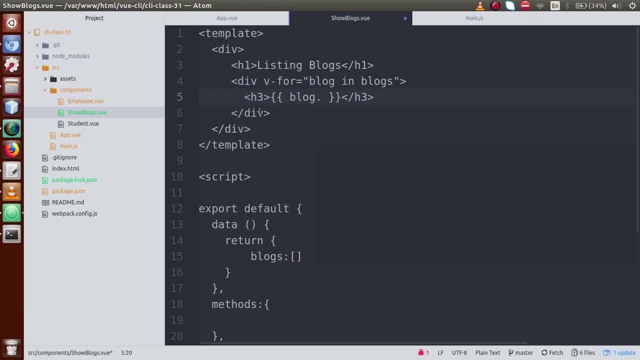 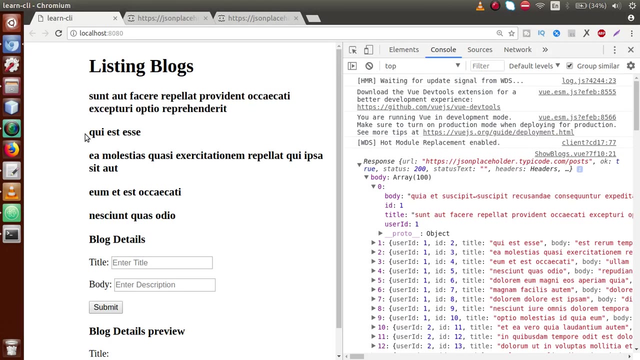 So something called blog. If I go to browser response page, so it contains a property called title. okay, So this is something called blogtitle. So just I will save it like this. just back to browser. And here it is, guys that we have retrieved the title through our fake JSON registry. 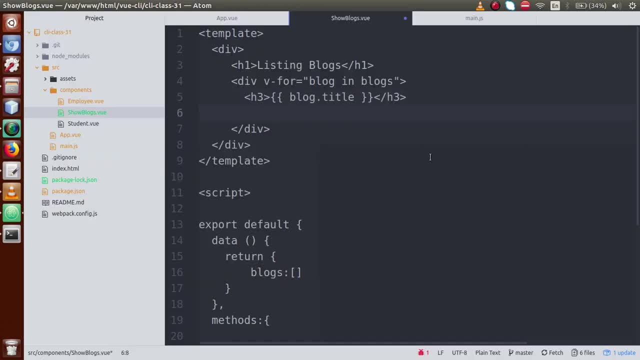 Okay. Next we have to retrieve, called the body section. So let's say that within paragraph tag, let's say that blogbody, or just back to browser And now inside this body as we have. okay, So blogbody.